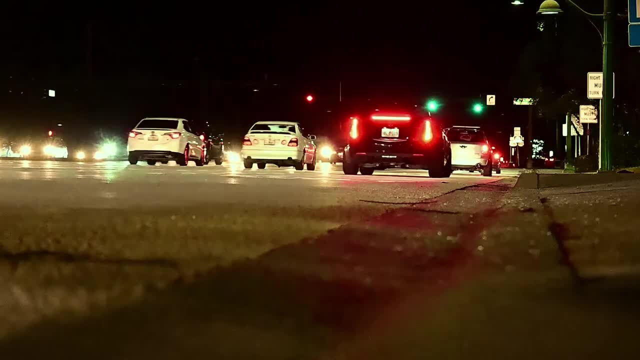 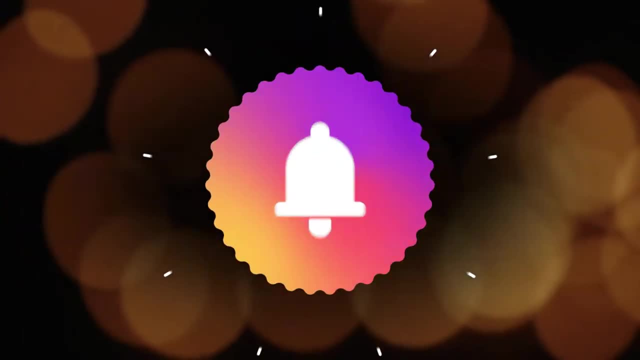 about accuracy in machine learning. Let's go to the content of how to increase the accuracy of machine learning model. So, before we start this video, do like, share, comment and subscribe. These things will help me to produce more new contents in Python and data science. Let's 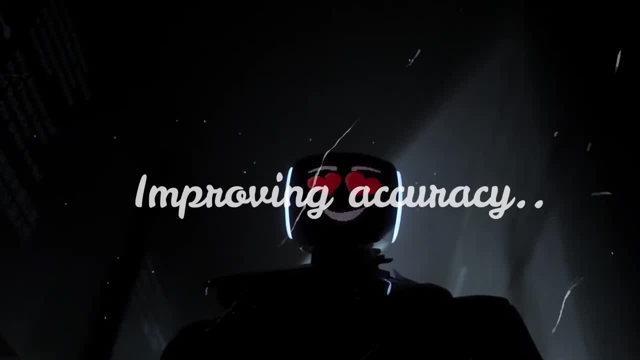 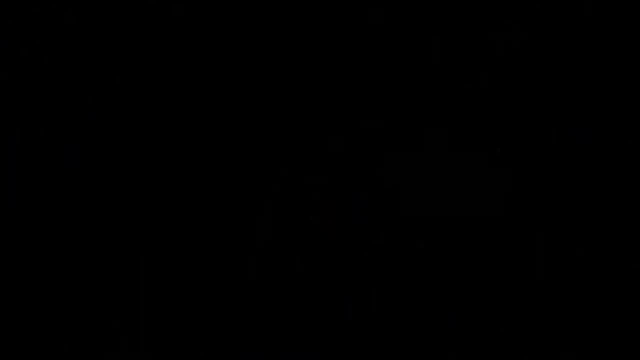 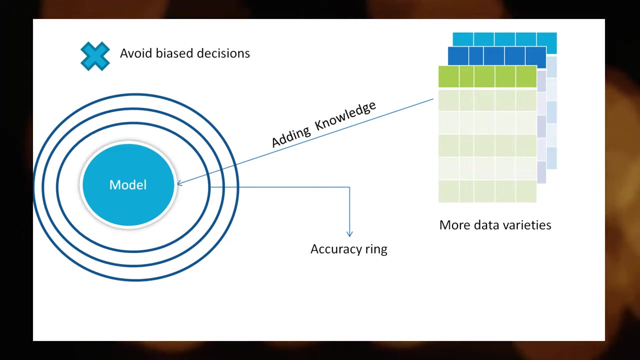 get started. First point is adding more data. Adding more data gives you more good and reliable results in the end implementations. By giving more variety of data to machine learning algorithms like you are adding more knowledge to the machine learning model, So it will get trained. 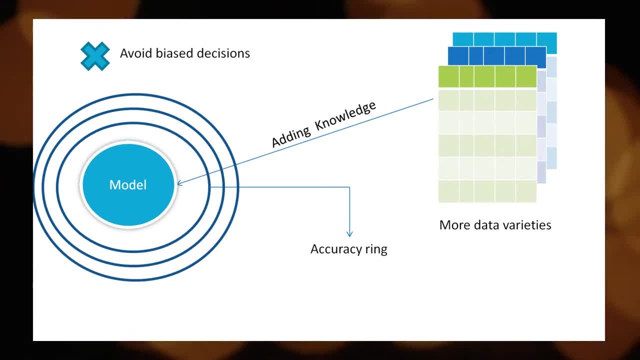 with some various data circumstances and it makes the model to do some comparisons before giving an answer. By adding more data, it will avoid to make some biased decisions And that means it takes super accurate decisions when it is deployed into the server or software. 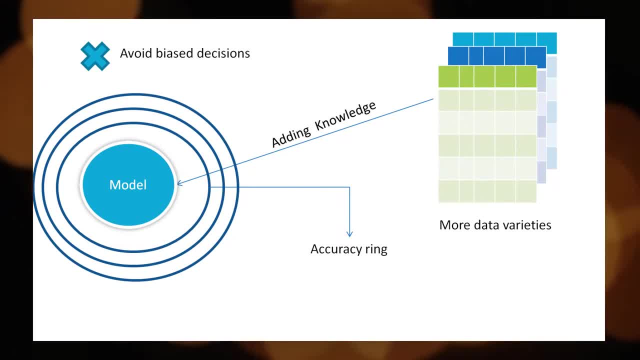 Suppose you have limited number of data and you trained your model with. that data means you cannot expect a good result At the end of training. in testing phase, your model will give you less accuracy and maybe you will get the results which are completely. 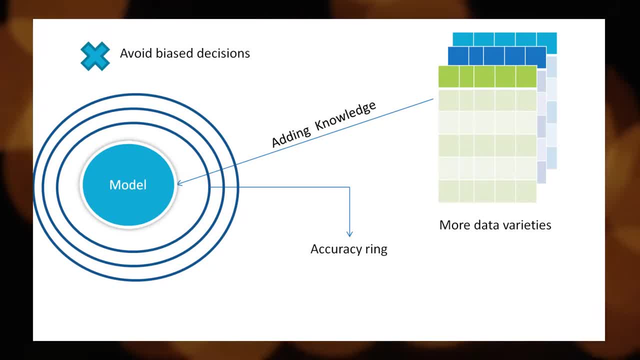 irrelevant to your expected results. So this is what a data plays a major role, and more data you add, more accuracy you will get. This is the tagline in machine learning, And second one is a feature selection. Feature selection part is very important in machine. 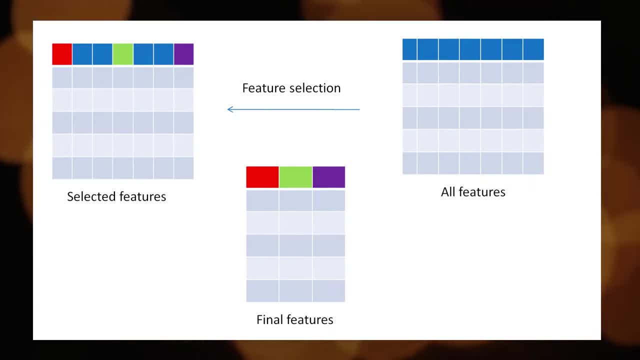 learning. So in this part you need to select the features that will create impact on your end results. Adding more data is a good, but in the data you have to select the features which will give less variance in your predictive model. If your variance estimation is high, then 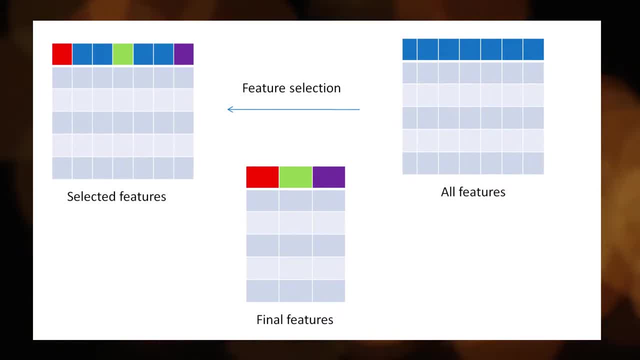 you have to drop some features from the training part. By reducing the non-impacted features in your data matrix, it will help you to reduce the variance and it is more advisable step to drop some unwanted features from your dataset. And one more thing: if you select, 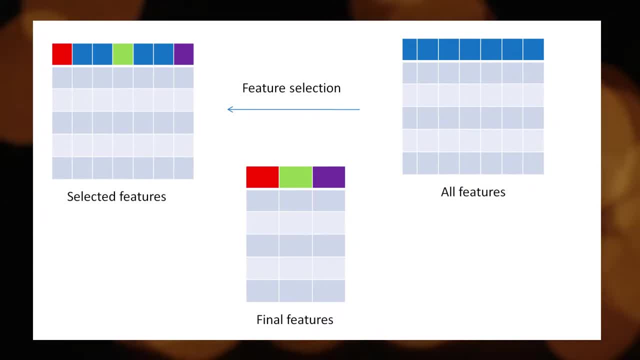 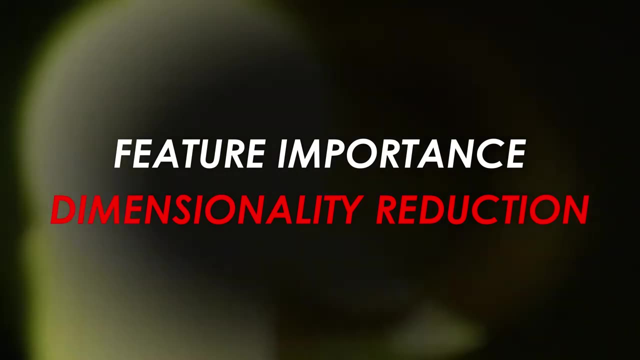 more relevant features and feed them into your model, you can avoid overfitting results also. So in this step, I will give you 2 important methods to follow while selecting the features. One is feature importance. Some algorithms, like random forest or XGBoost, allow you to. 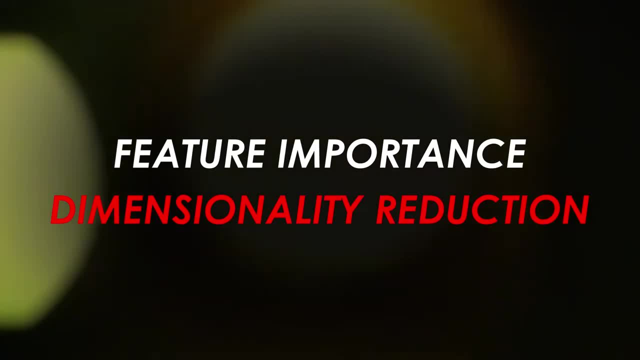 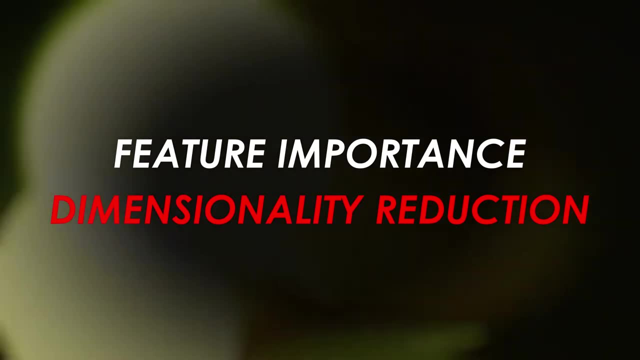 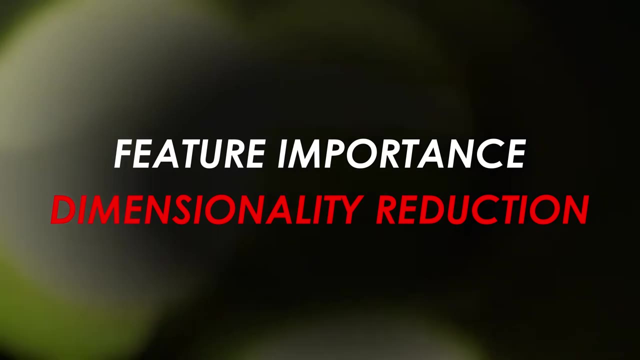 determine which features were the most important in predicting the target variable's value. By quickly creating one of these models and conducting the feature importance, you will get an understanding of variables are more useful than others. okay, and second one is the dimensionality reduction. one of the most common dimensionality reduction technique is the pca. pca means principal. 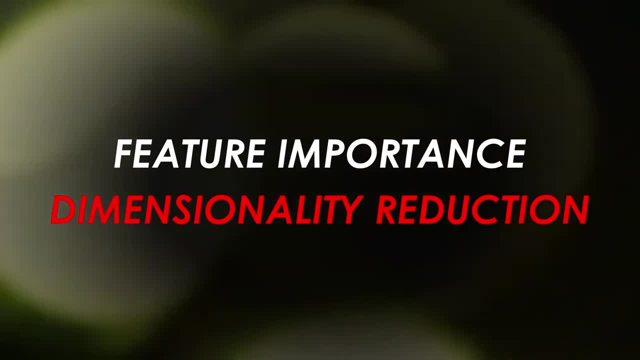 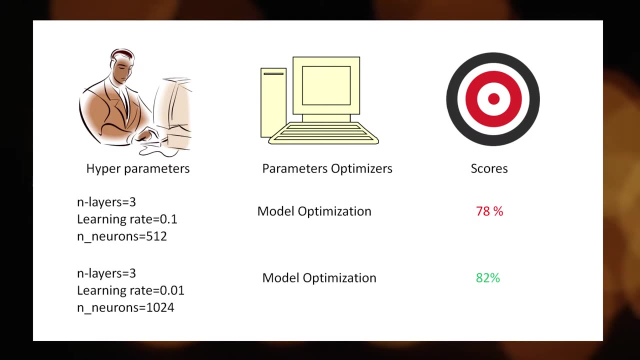 component analysis. it takes larger number of features and uses linear algebra techniques to reduce them into a fewer features. and third point is hyperparameter tuning. training a machine learning model is a skill that will come if you practice more in problem solving. and sometimes these above techniques are not enough to improve the accuracy of your model. 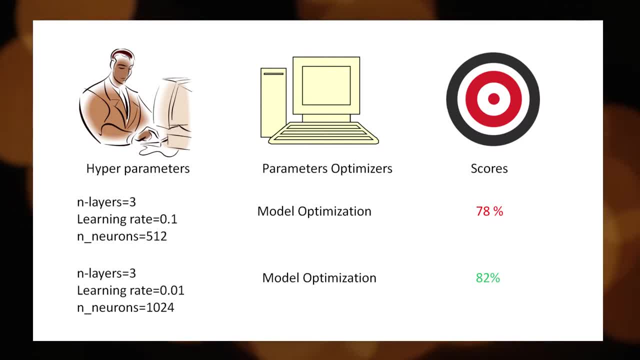 so in the field of machine learning there are a lot of techniques you have to follow to increase the accuracy of the machine learning model. you can't able to stick with a particular technique to improve the accuracy of machine learning model. one of the best way to increase the accuracy of 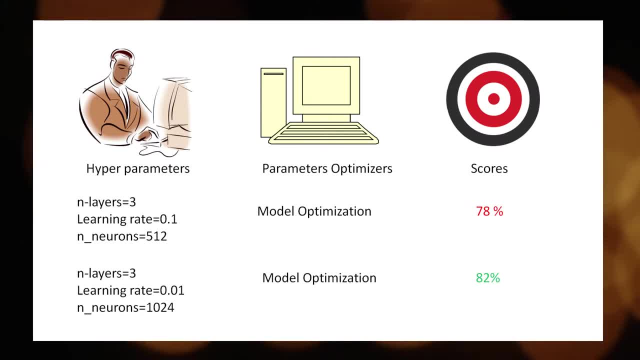 machine learning model is by implementing the hyperparameter tuning in your model. so it is like a trial and error method. you have to change the model parameters until you reach some good results and accuracy. So this is the strategy that is followed in the hyperparameter tuning. 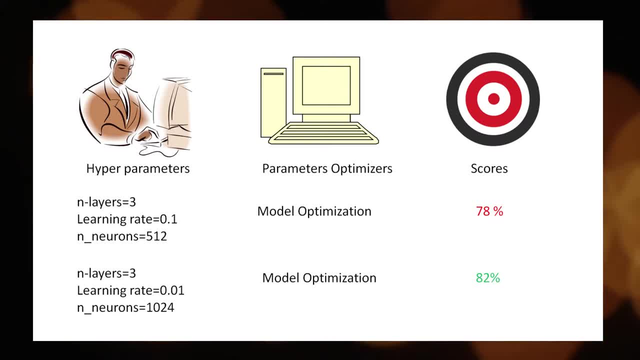 Hyperparameter tuning is more important in unsupervised learning. So take an example: when you are training the k-means algorithm and you don't know how many clusters to add. In this case you have to change the cluster values until you get some good accuracy. 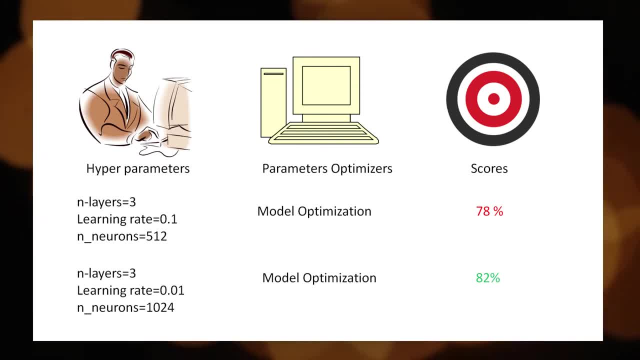 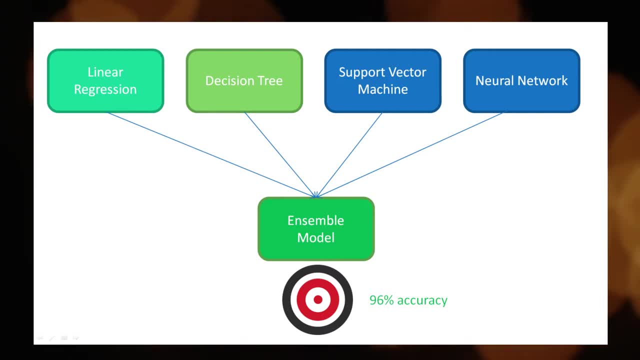 We already made a video about the k-means clustering in our channel. If you want to understand the k-means clustering means, you can go and watch that video. And the fourth one is the ensemble methods. This is one of the most common method which is used by every data scientist. 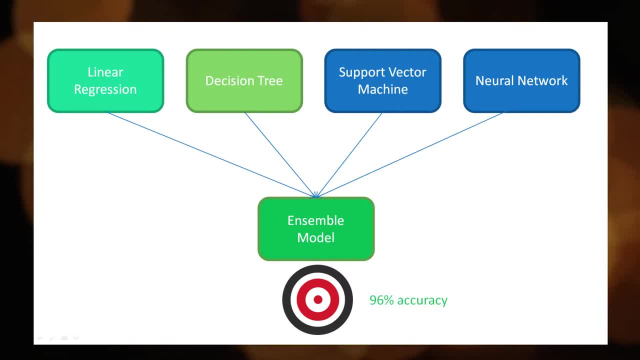 Suppose, if you are hearing the ensemble words for the first time. So this is the explanation about the ensemble methods. Ensemble methods are nothing but combining the multiple trained models and produce a good accuracy at the end. So this is the process of ensemble methods. 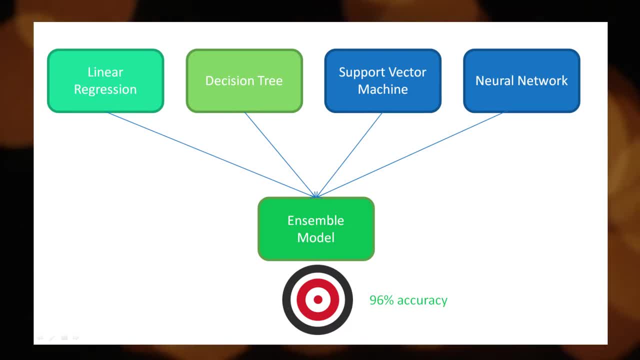 Ensemble method is a winning strategy of every data scientist and machine learning engineers. This can be achieved through two common methods. The first one is the bagging And second one is the clustering And third one is the boosting. So I am planning to create a separate video for ensemble methods in machine learning.